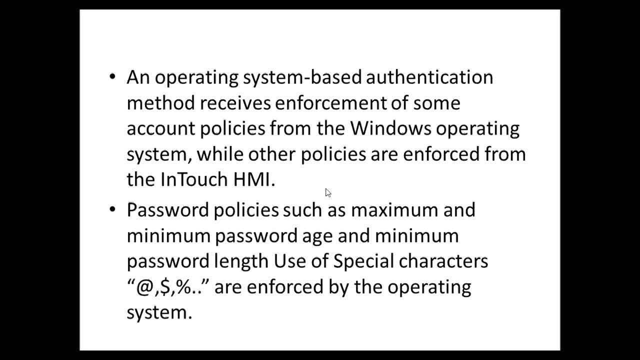 enforced from in touch HMI. so what is that? what do you mean by Windows operating system policies? so these are the policies which are actually applied by the internal IT of your organization to your user username and user password, your credentials. so let's say, assume one example: whenever you are joining any organization, the IT will 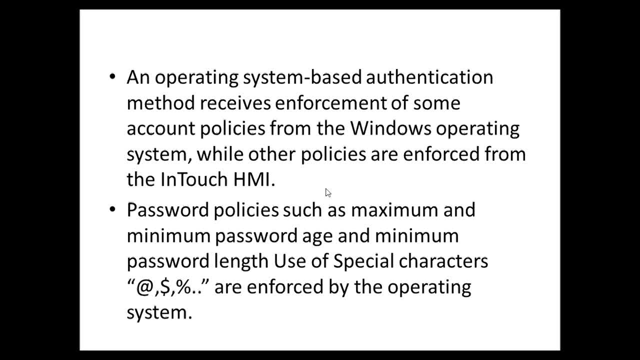 provide you login credentials for your system, which may be the profile login. you can use that login in any of the system. okay, this is basically Windows password that you use to log into the system. so IT can restrict or apply the password to the system. so it can restrict or apply the password to the system. 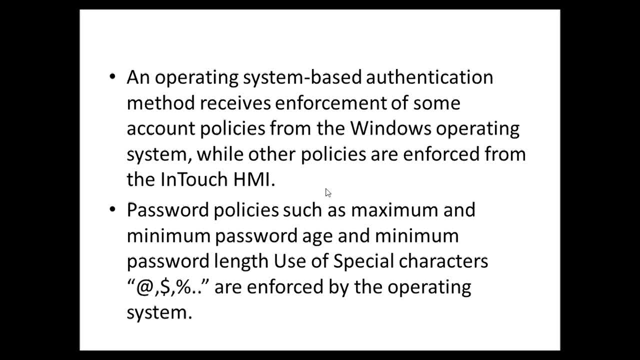 policy or the passwords, like: maximum number of days to change the password should be 45 days means the system will enforce you to change the password or the password length must be within minimum of nine characters. it should contain special characters like at the rate dollar percentage within the 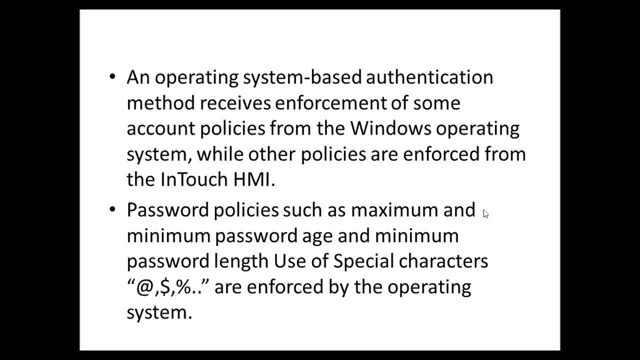 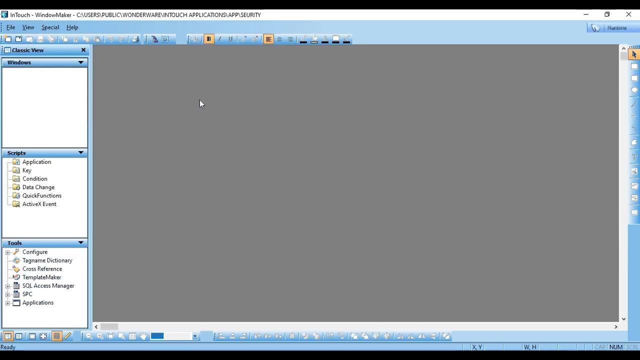 password, like, likewise a, so IT can change the group policy and apply some of the policies to meet the customer requirement and IT compliances. okay, so basically in this type, user credentials are controlled by IT, some of the policies are controlled by IT. so let's develop one application using Windows security. 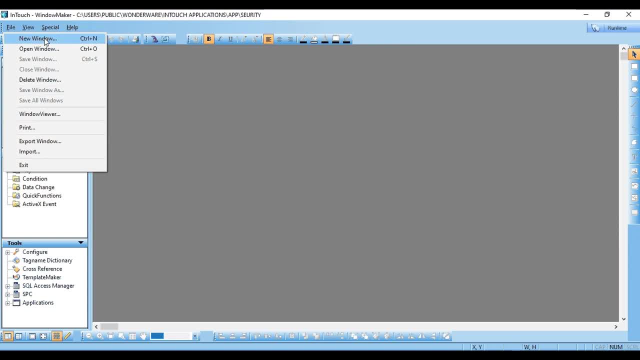 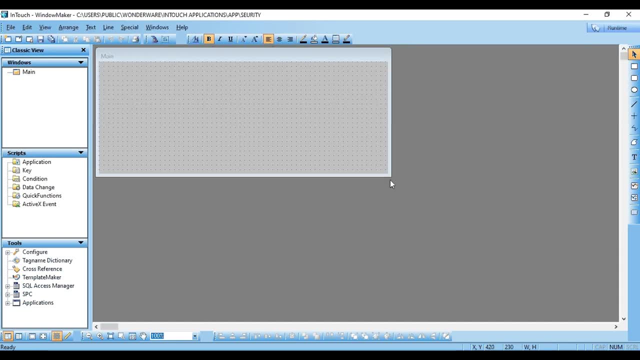 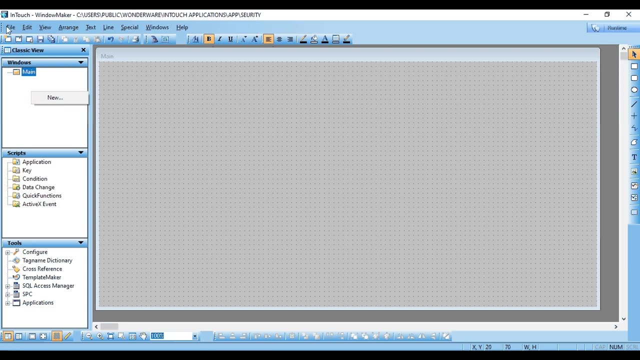 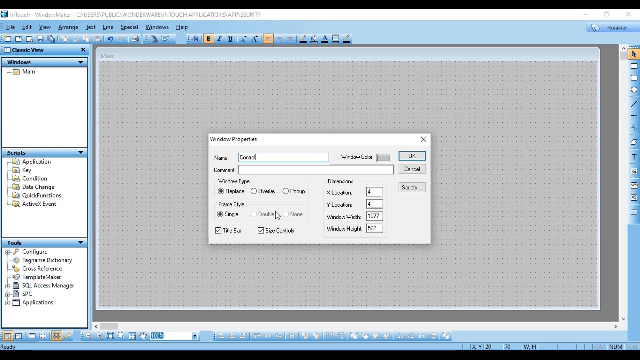 okay, so first of all, we need to add some windows. it is main window and let me say, control window. let me add third window and let me add third window and let me add third window and let me add third window, which is emergency window, which is emergency window. 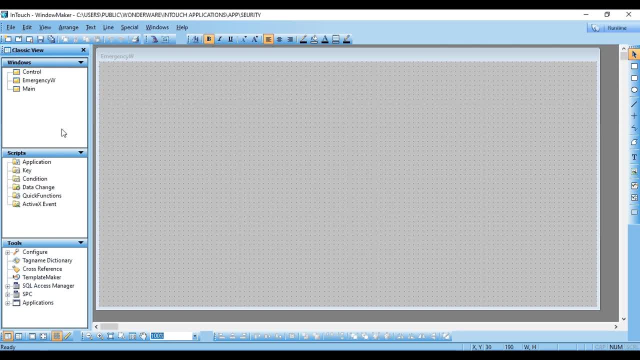 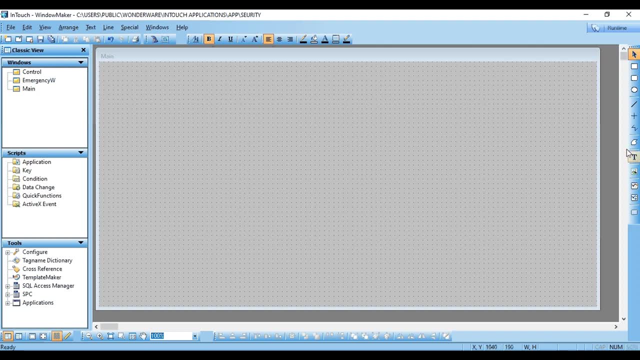 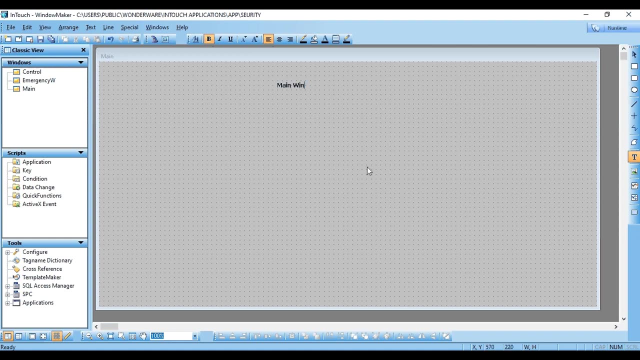 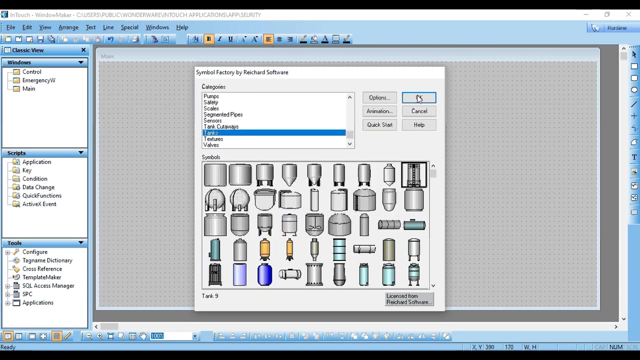 emergency. okay, so on my main window I am adding: let me just a title this window main window. okay, so just call this one main window. this is lunch slash coffee place, IE. what type of coffee is it? probably I have added not just to avoid any confusion. Let me add: We are not going to add any animation to this. 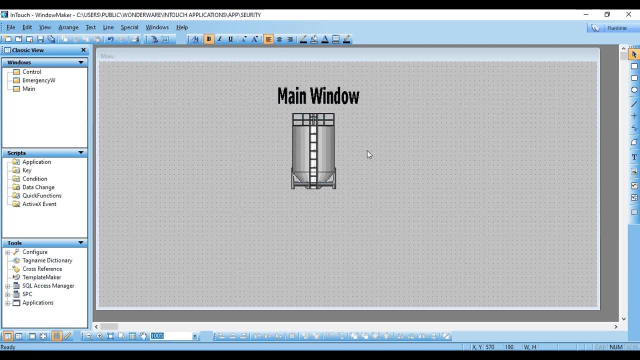 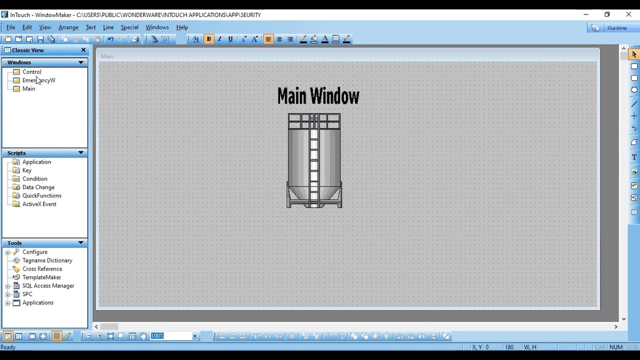 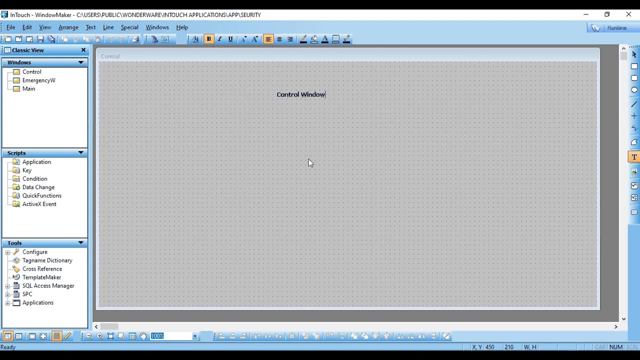 tank, but just for clear visibility, I am adding this, I am adding some control window and emergency window, Okay, Okay. So again, we're going to main window. Now, before applying, before enabling Windows security, Let me first make two concepts very clear. 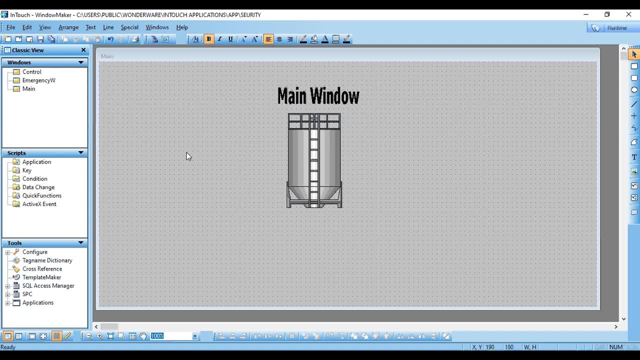 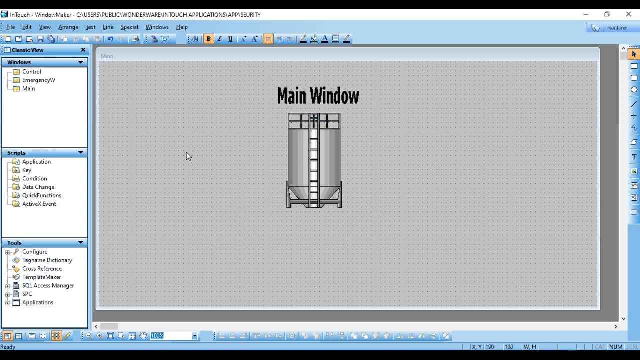 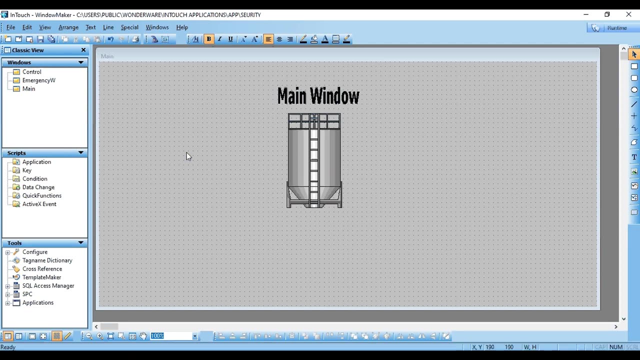 So authentication and authorization. so what is authentication? authentication means we are identifying, we are recognizing valid user, the user which are allowed to use this application. and second, authorization, authorization means determine- we are determining the privileges granted to authenticate user. that means, let's say an example, there are three users. one is 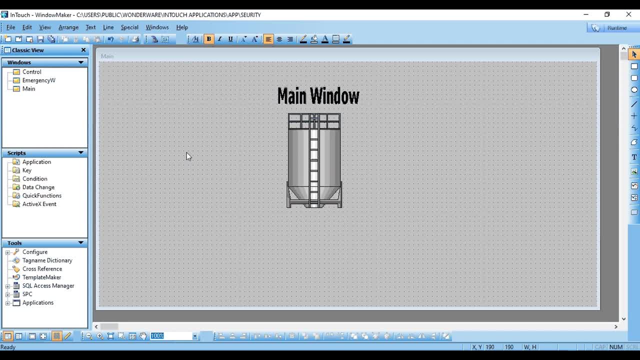 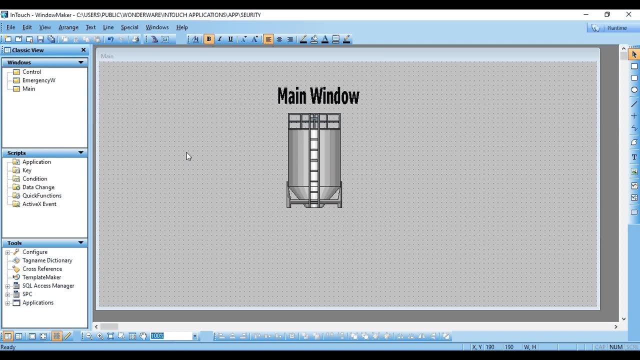 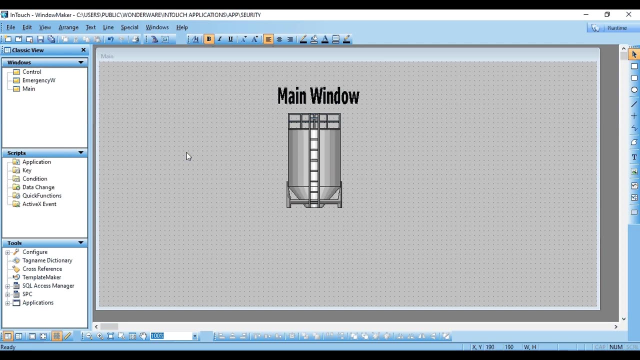 operator, second one is the actual engineer and third one is the person who is highly qualified and very responsible, which has, who can have, maximum rights to access the application right. so access level should be different for all all the types of all the category of the users. okay, 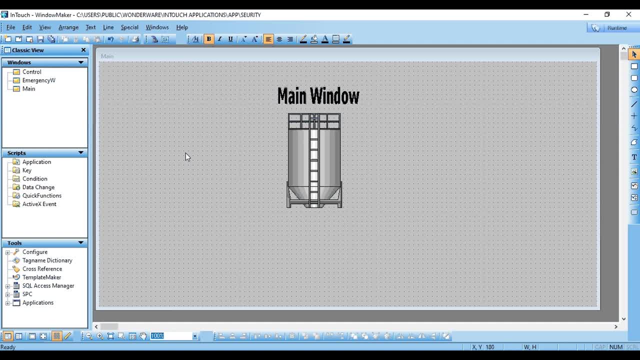 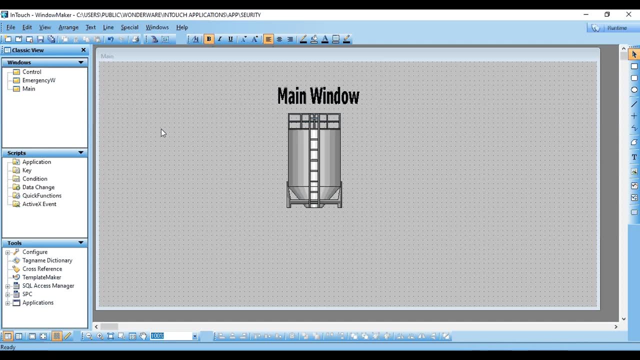 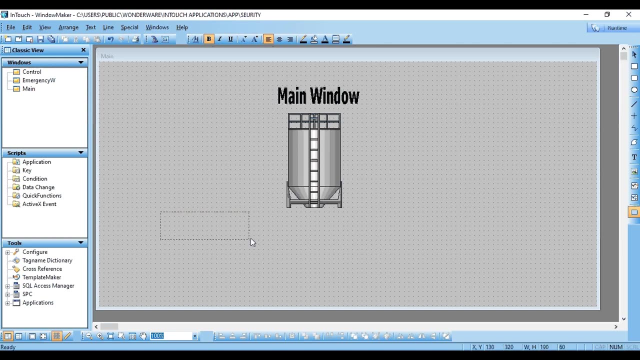 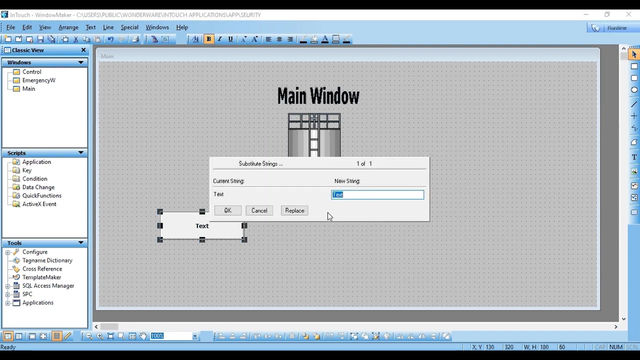 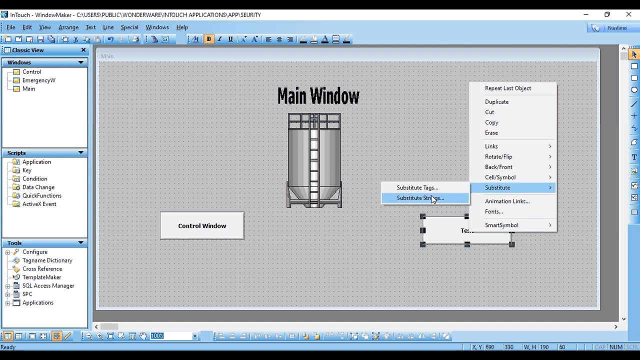 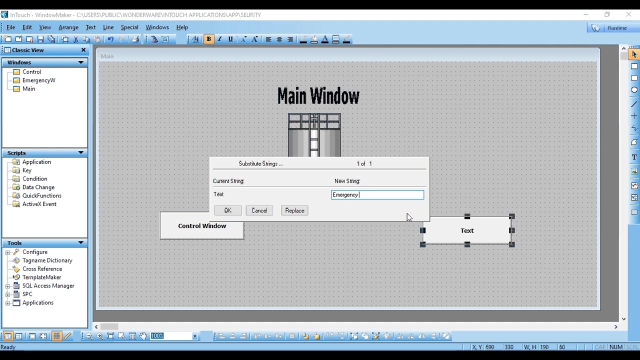 so we will see. we will encounter access level also in this in the coding, okay, so hope this is clear. so let's add the button substitute: string control window. okay, that may another button: emergency window. okay, so now let's first. i have added two button. now my purpose is the person who has the access. 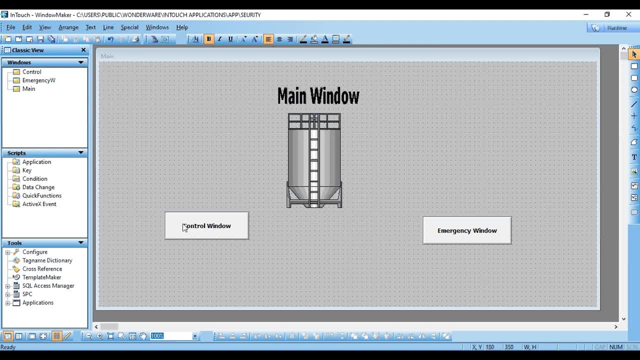 to the computer first, let's add one button first of all. let me add two buttons to the computer here and you can add. if you click on add two buttons to the computer here, you can add any of the the access level to control the window, to actually access the control buttons. 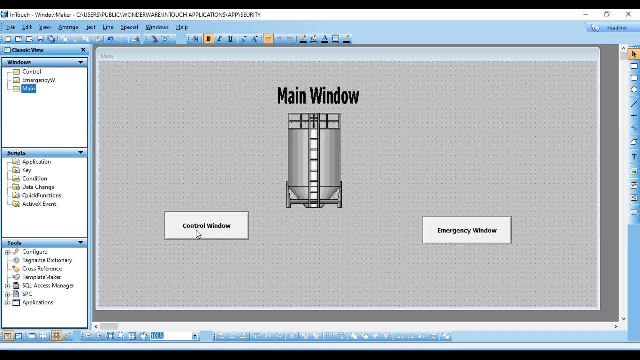 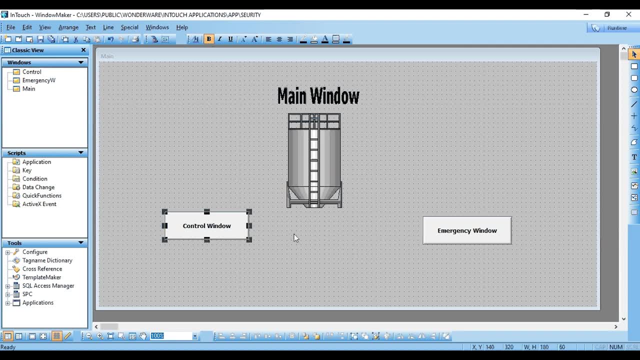 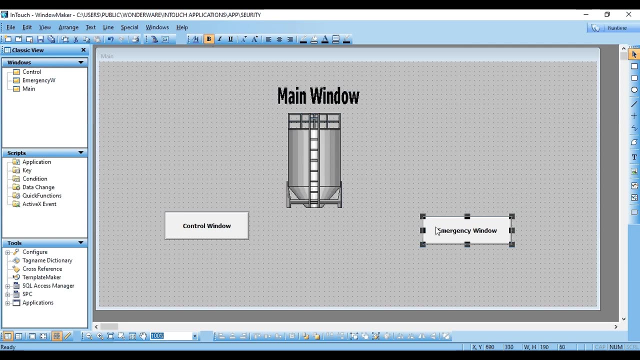 over this window can only see this button- control window- okay, otherwise it should be invisible, disappeared, okay. and that person who has the rights to view emergency window can only see this button, otherwise it should be invisible, okay. so now I am very first time adding the access level, now for Windows. 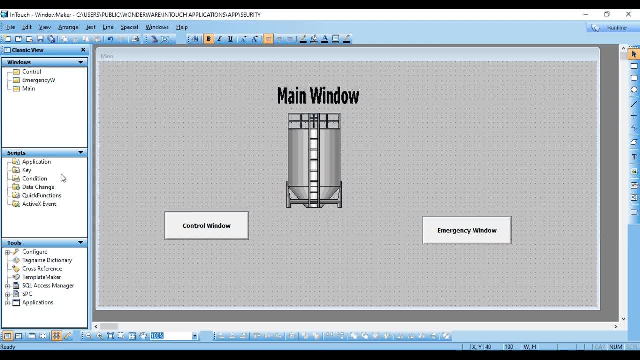 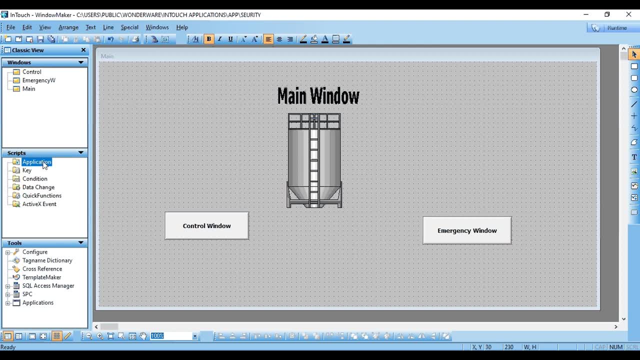 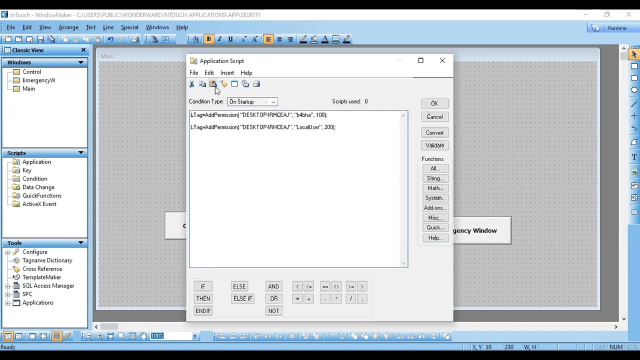 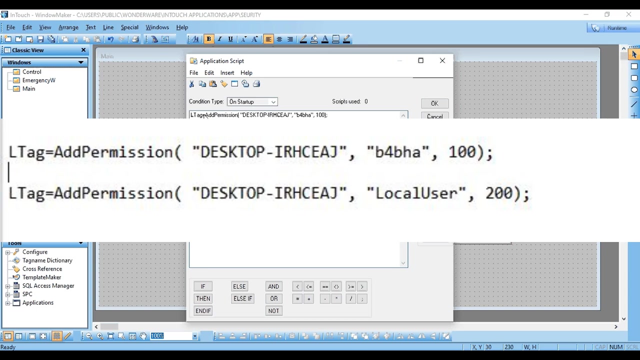 security. we need to add the access. so I'm going to application script in script. ever click on application in application script, select condition type. only start up. I have just added the codes to add permission, which is a tag. you can define any tag here, any tag name, it can be anything equal to add permission in. 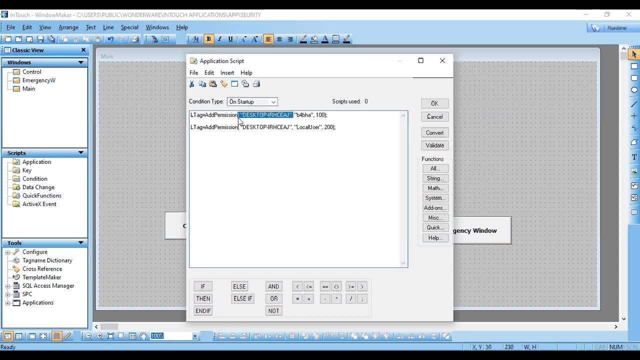 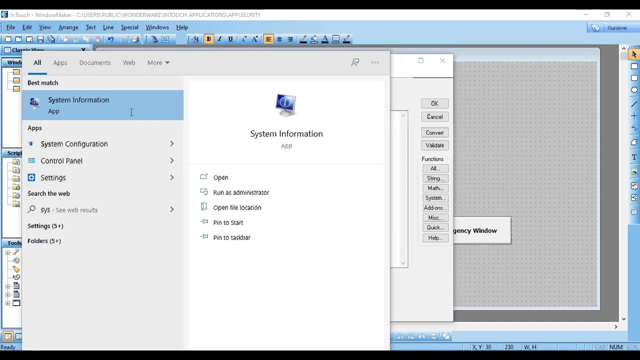 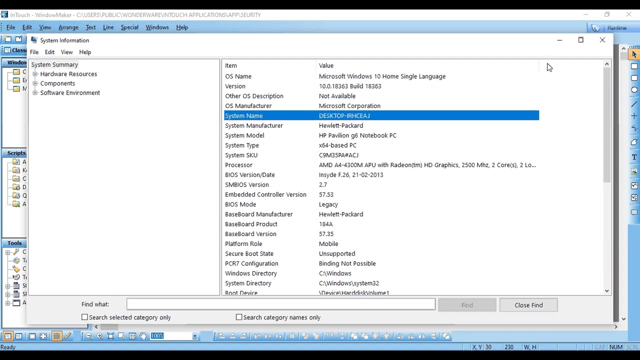 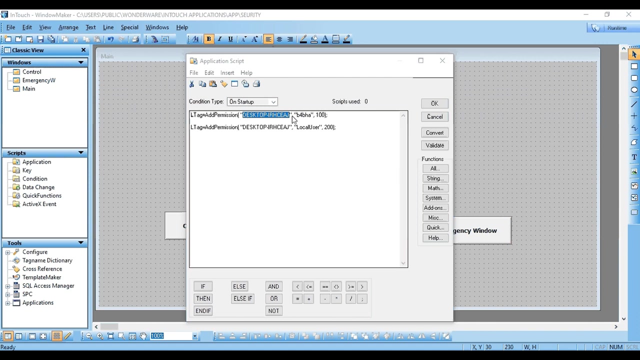 the bracket now. first one is: should be a domain name or your computer name. okay, so I have just added my computer name. okay, so it should be available in your system information. so this is my, since the system in system name on this system information. so I have added system name comma. this is the user name, okay, 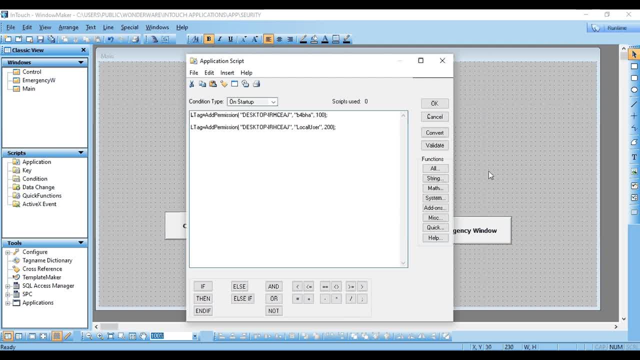 which we use as a user name for our win, to log in our window or to log in our profile. okay, so this is my username and my access level is 100. okay, we will see in late. we will see later in this video how to use this access level. okay, and I? 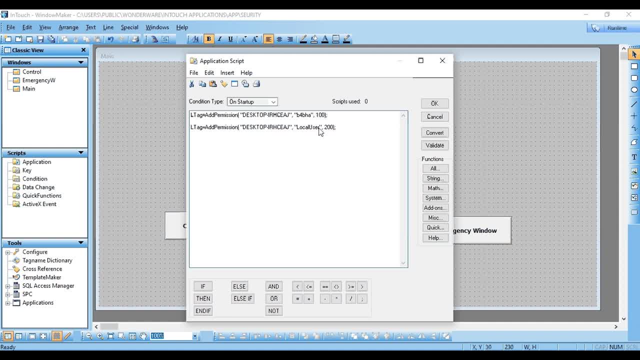 have added this another user which is local user. okay, so make this user a local user. okay, so make this user a local user. okay, so make this user a local user. okay, so make this very clear. I am NOT creating any user. these are the already available user on my system. okay, so you need to use the username of your windows, so for 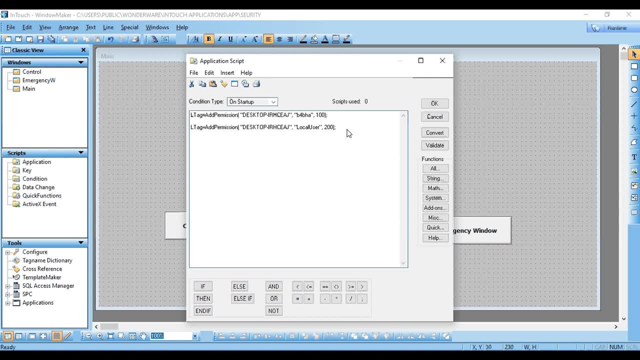 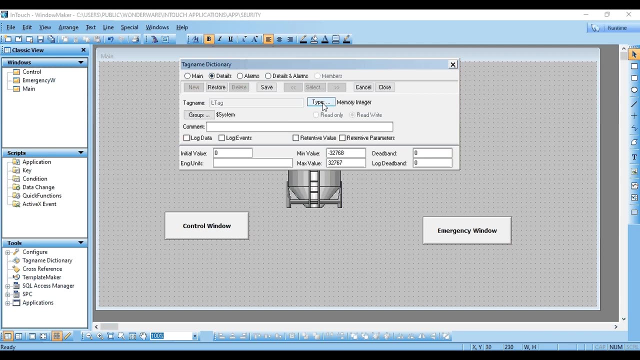 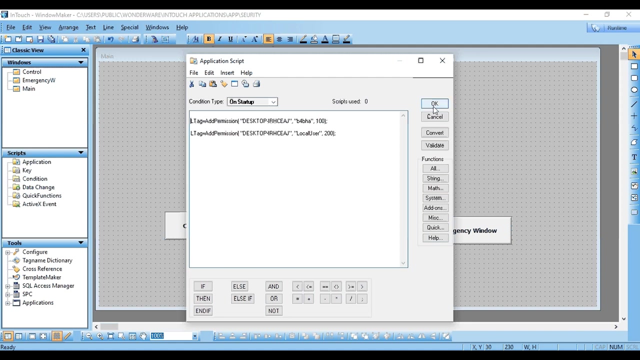 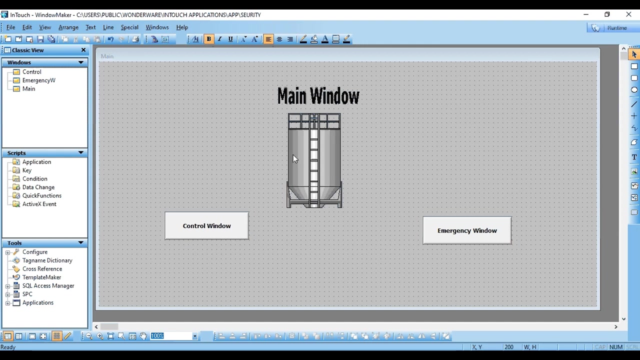 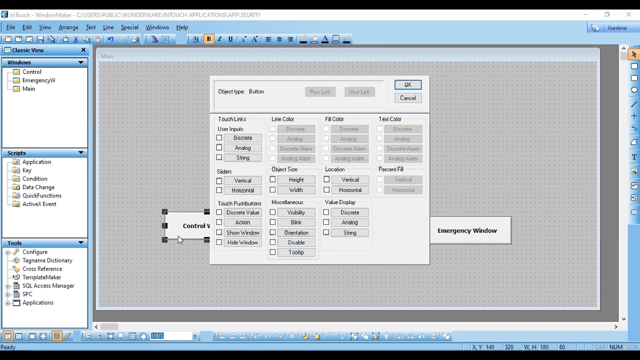 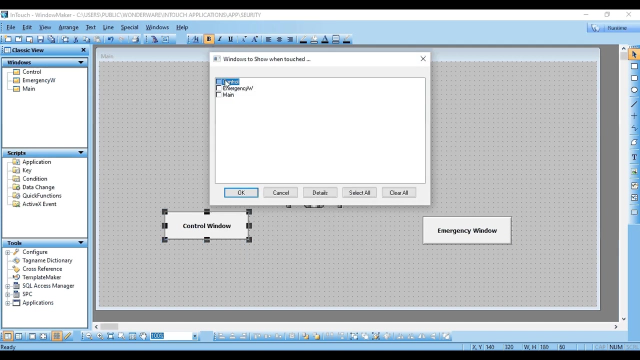 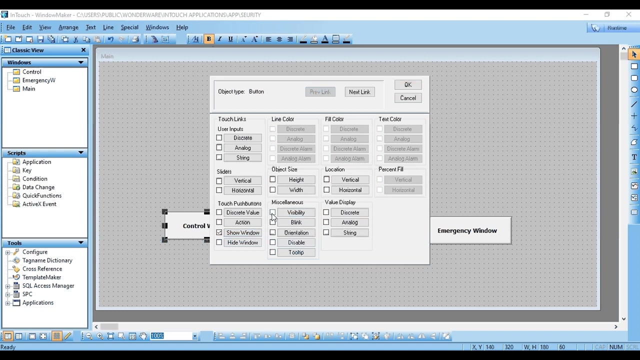 second user, my access level is 200. okay, now this is asking me to define the tag name I. I have just see you here. now 창, the control window, what we are, angle window and I control window. so selecting the control window, okay, and visibility. so if the access level is 100, 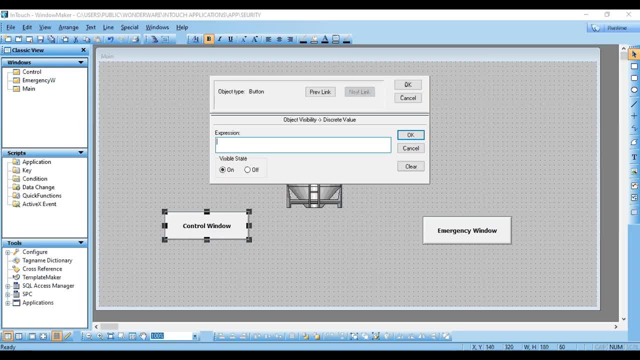 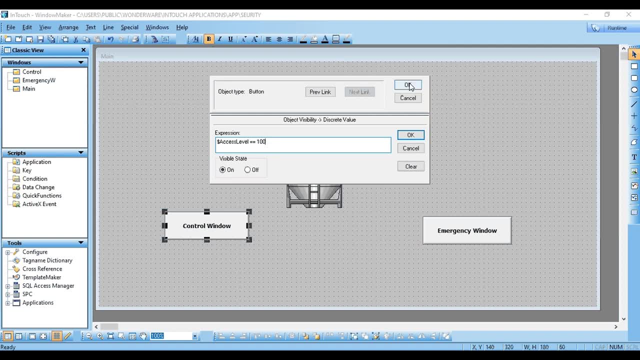 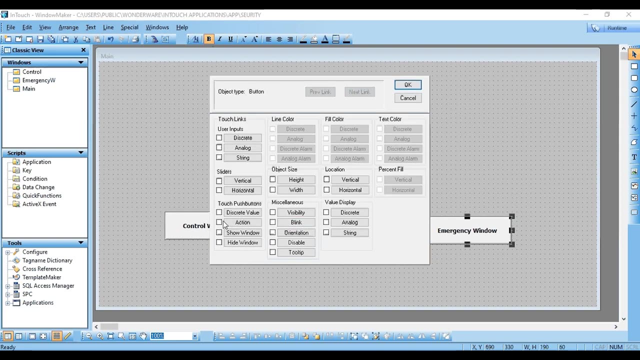 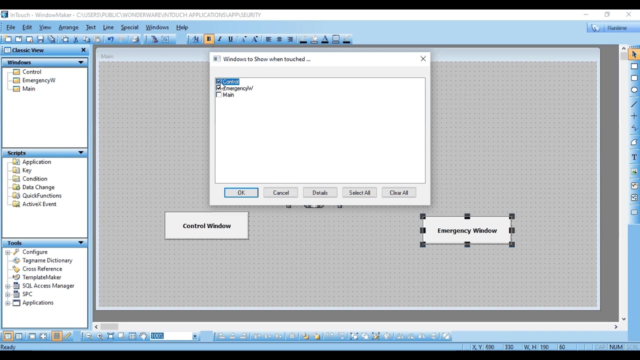 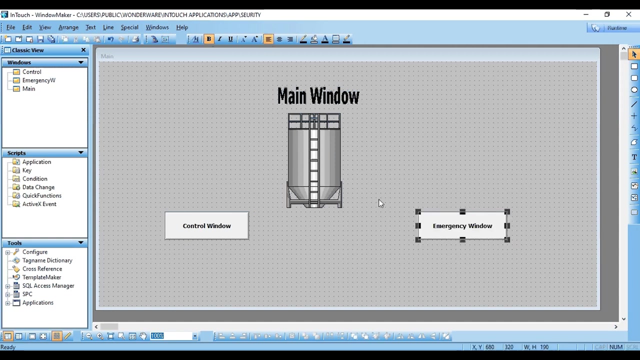 then only this button should be visible. so i have added dollar access level equal to 100. okay, same for emergency window, what we want it should show emergency window, okay. and for visibility, access level should be 200, okay, yeah. so now let me assign, let me select the type of security. so from this special menu, security, select the type. 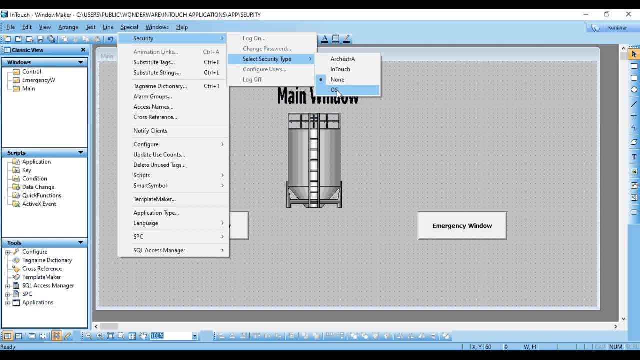 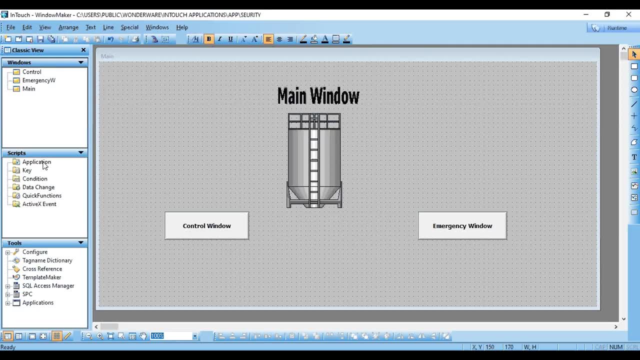 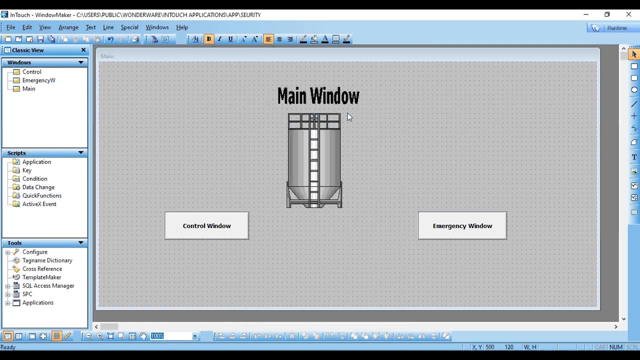 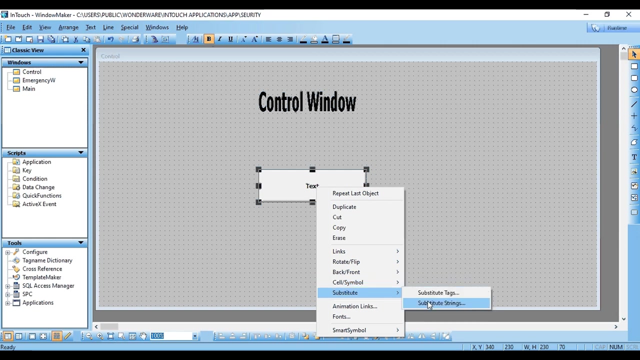 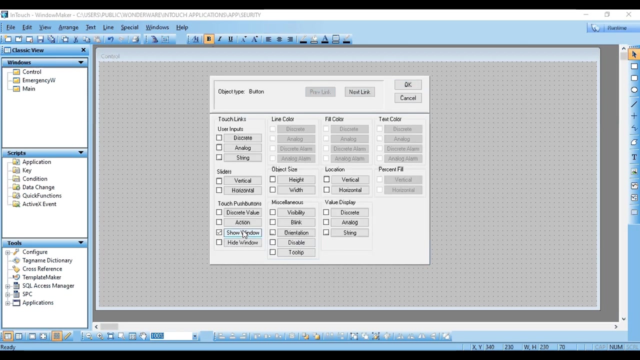 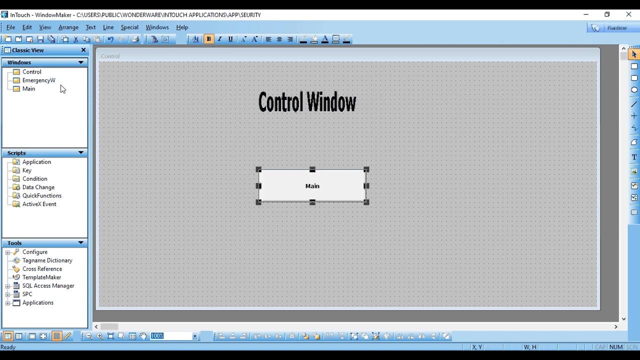 security type to os, because we are working for windows security. so select os. we have already assigned the access level in application, okay, so now let's check. just i want to add that return button on this window to move back to our main screen. same for emergency window. 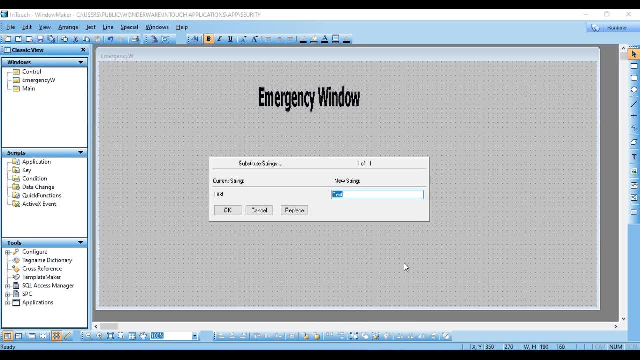 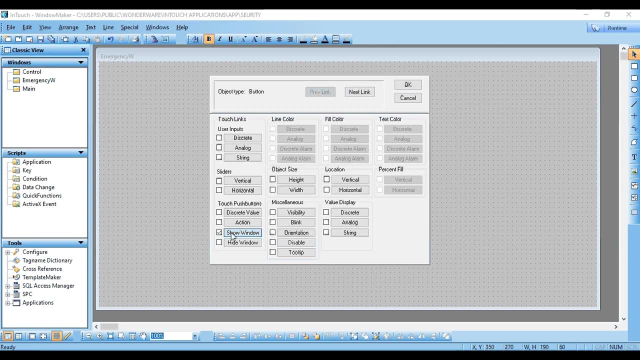 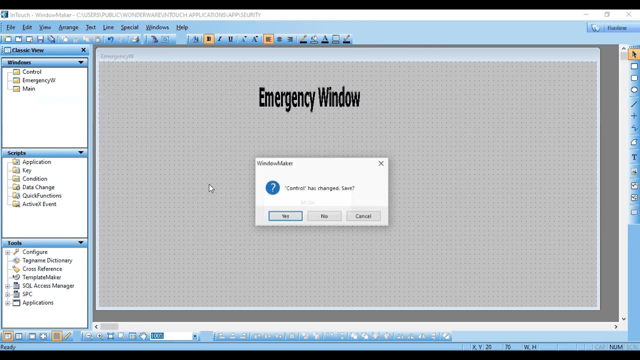 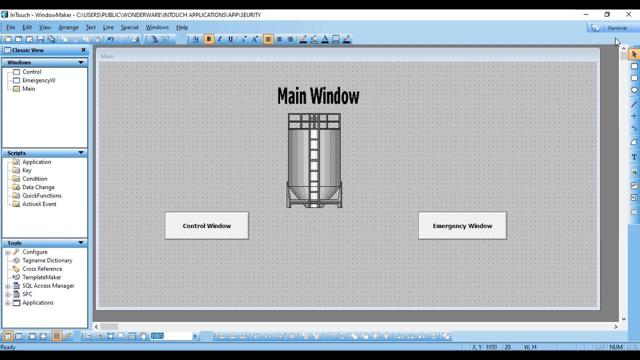 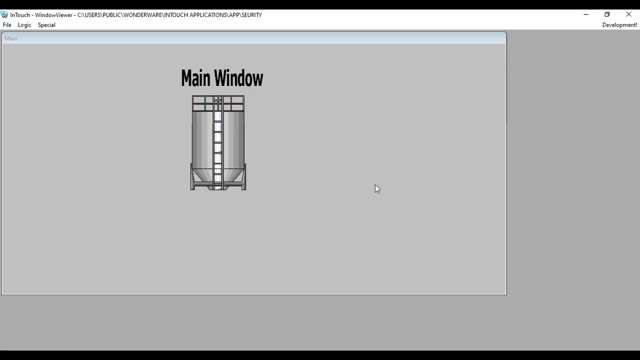 so okay, we are done. so okay, let's check. so, as you can see, none of the buttons are visible because i have not logged in as any user. now click on special security logon. now let me log on as b4bhu. this user has access level 100. 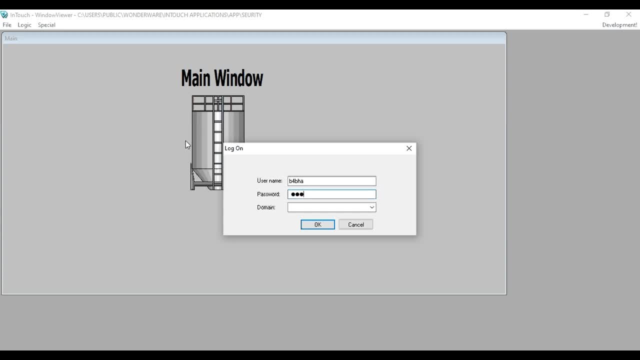 i am entering my system password, my laptop password, okay, and my system name. if you are working on network system, then you need to select the appropriate domain. okay, i am working on my local system. okay, so my access level was 100, so the control window is only visible. the rest will not be. 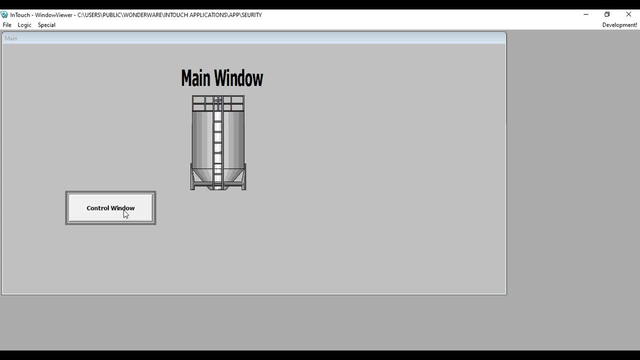 will not be visible. so in this way you can protect any of your window appropriately from the access level. so by clicking I can see the control window. okay, going back to the main window, let me log off. okay, so button is now not visible. let me log in. and another user, just local user. 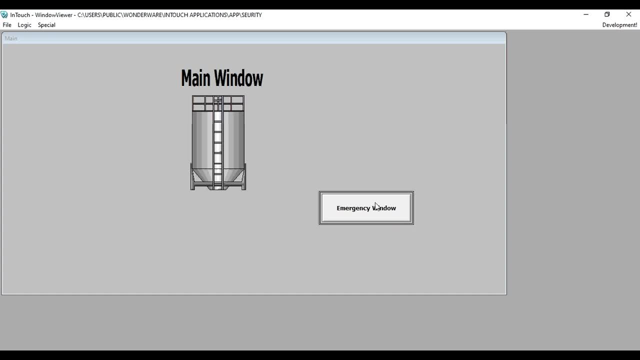 okay, so now emergency windows button is visible because the access level of this window, this button, is 200. that's why it is visible. okay, so this window is now secure. now let me cover another point, which is timeout. so now, suppose, if I have login for the emergency window and I am just 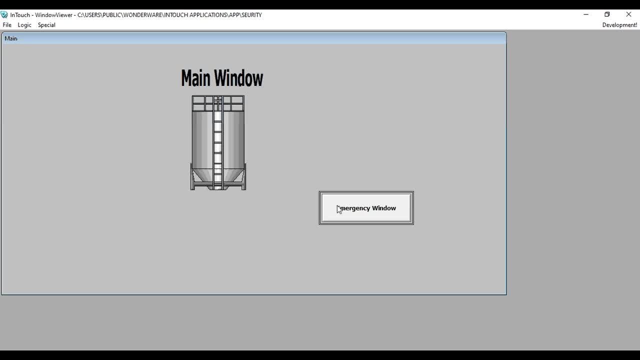 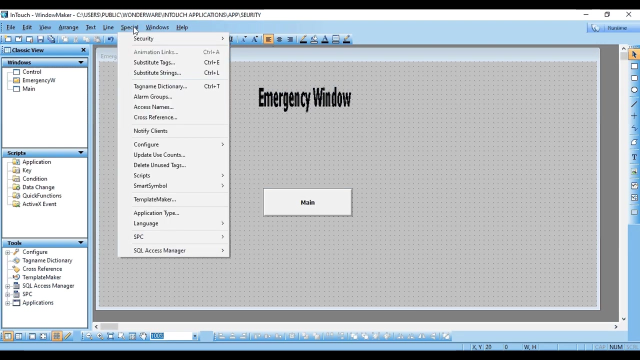 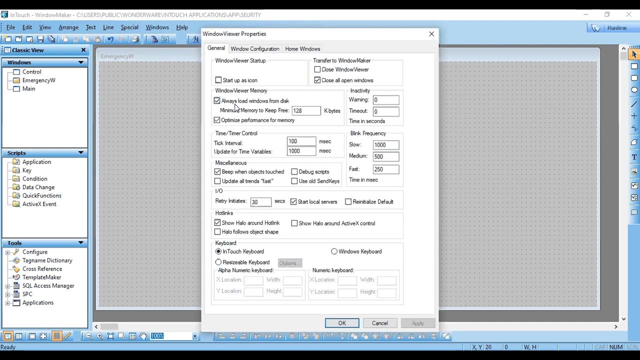 moving, a moving from my desk, so it may be critical to protect the unauthorized access from the system. so there is one feature which is timeout, so it can be added from special configured Windows viewer. here you can see in activity in activity okay, so you can assign this. timing will be in seconds, so be careful. I'm just. this is just for. 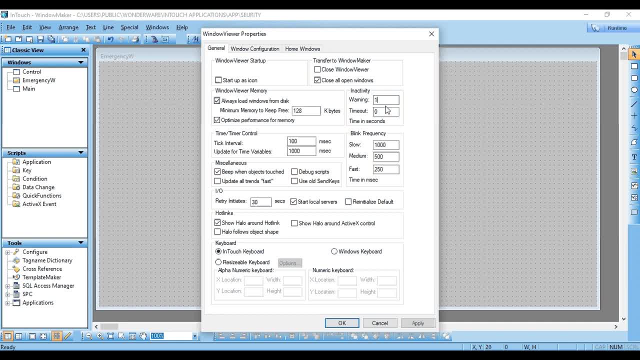 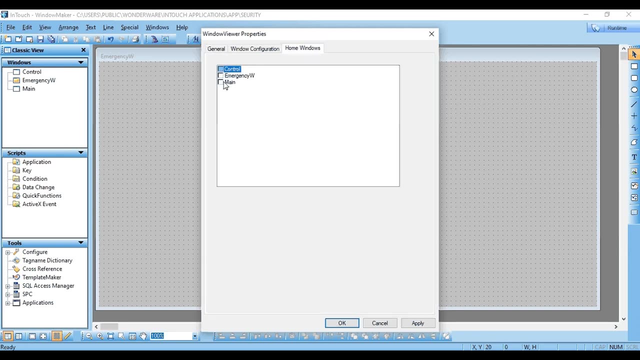 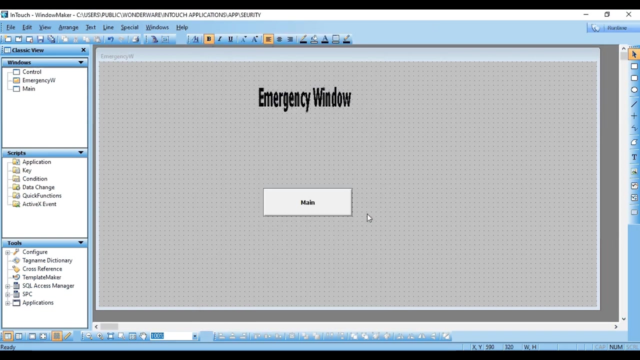 demo purpose. so I am adding 10 second or 20 second for warning and 30 second for timeout. okay, let me select. this is just for main window. it is getting me to restart window viewer so I need to close the window viewer. okay, so I just want to add some codes to control window if the system is identifying. 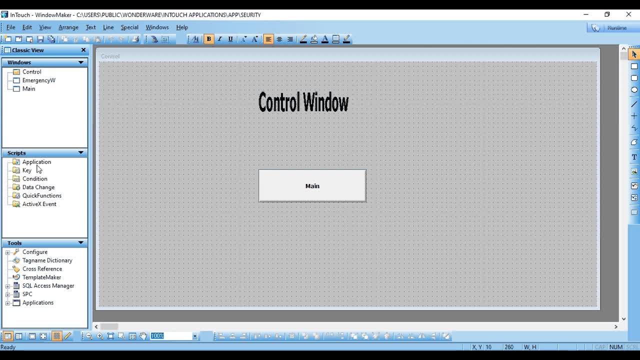 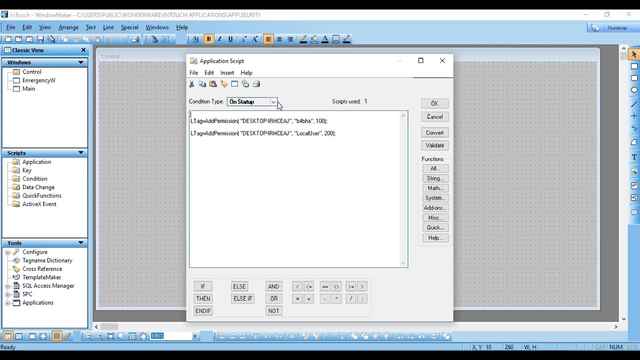 timeout duration is reached to its timeout or idle duration. okay, so open the application script while running. execute every 100, so if the access level is other than 100, then hide control. okay, this control window. hence, what does it mean? if I am, if I have logged in to the application and open the control window, but if I am idle? 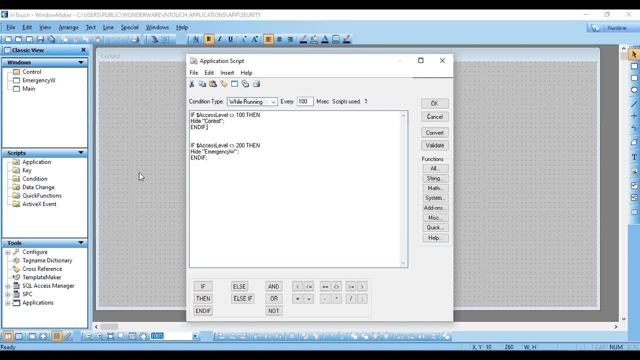 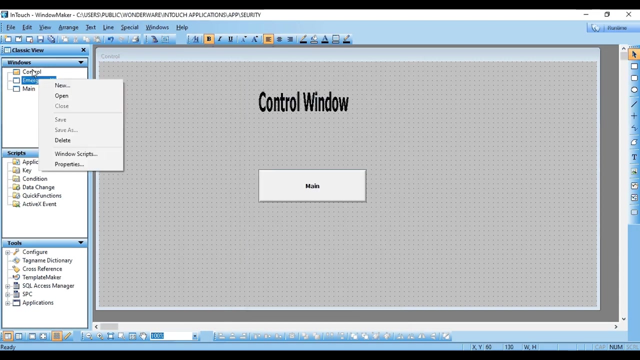 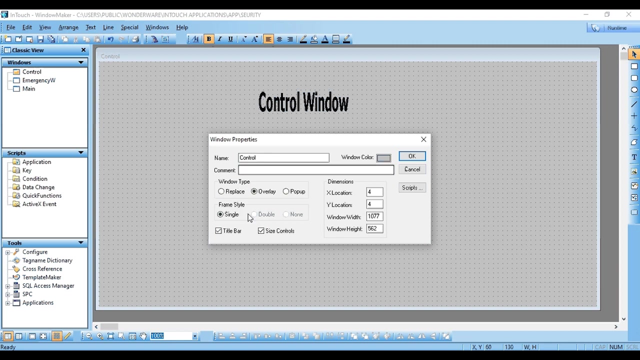 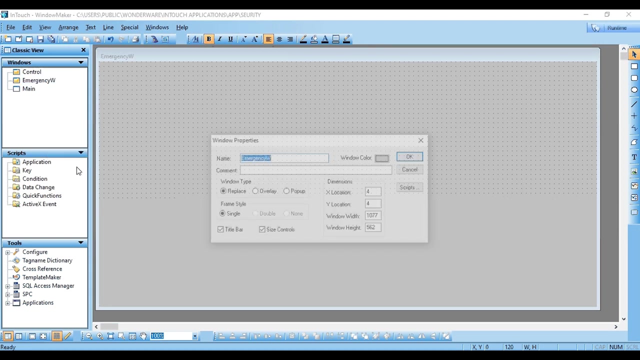 for the 30 seconds which is my time of duration, and this window will closed. okay, same for emergency window. if it is not adequate access you and windows we close. I'm just changing the type of my window following control overlay. it's not required, but just for the demo purpose it will be. 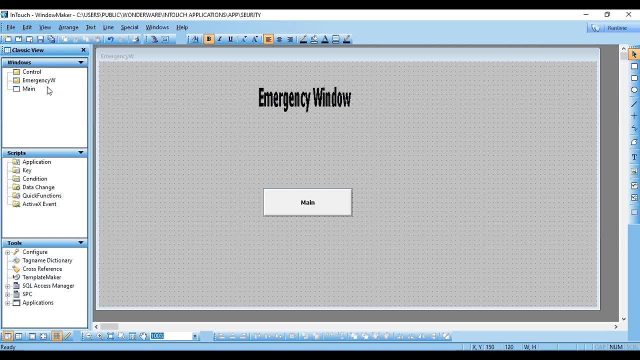 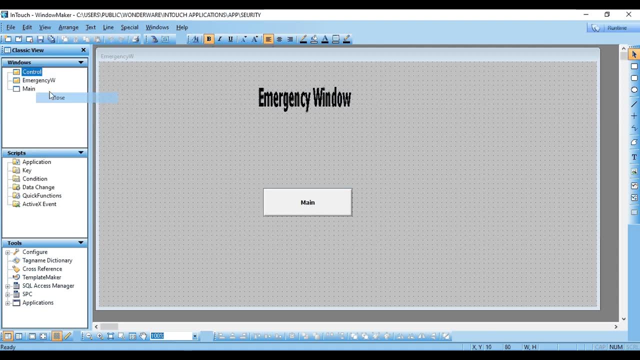 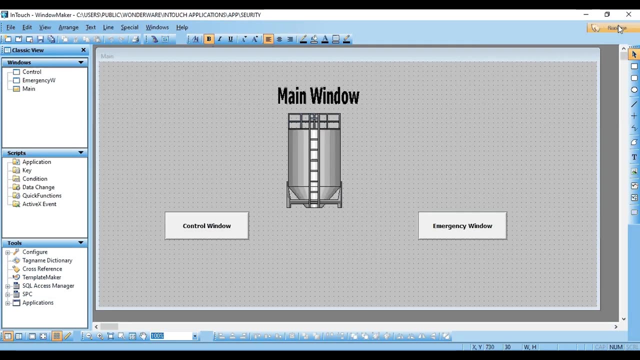 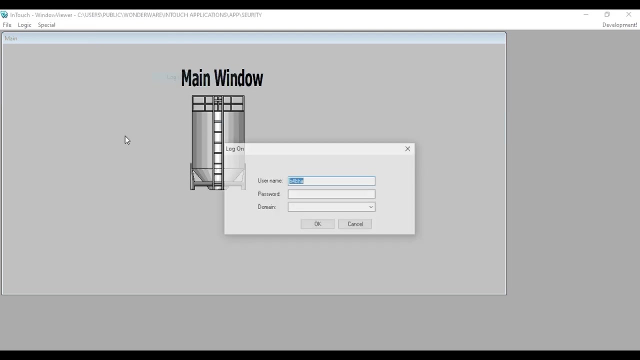 good, okay and close, going to the main, and let's execute. so none of my button is visible. now let me log in as P for PHA. okay, my control window is visible now. if I will stay idle for 30 seconds, it will be again disappear because I will be automatically logged off from this. 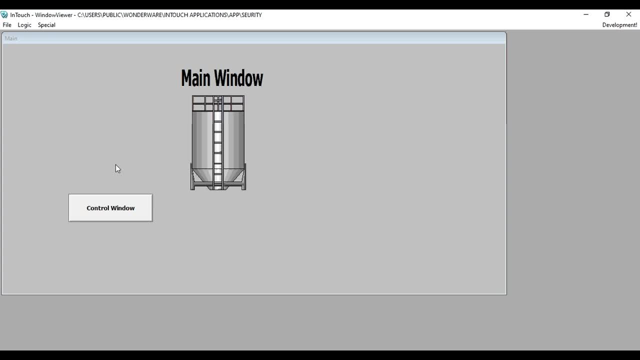 application. let's see. yep, so I have. I am automatically locked off due to timeout, so this is very important again, let me log in you now. I am opening control window and remember we have added that accent script to close that window for the ideal duration. it will not match the access. 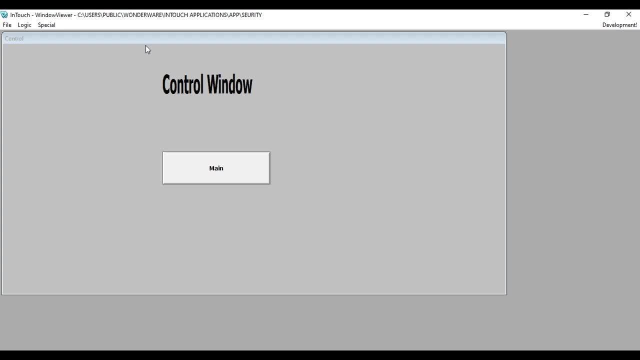 level, this window should be closed, so I am waiting for 30 seconds. okay, So, as you can see, due to the idle status of that window, for the 30 seconds I am automatically logged off and due to my script, that window was also closed. 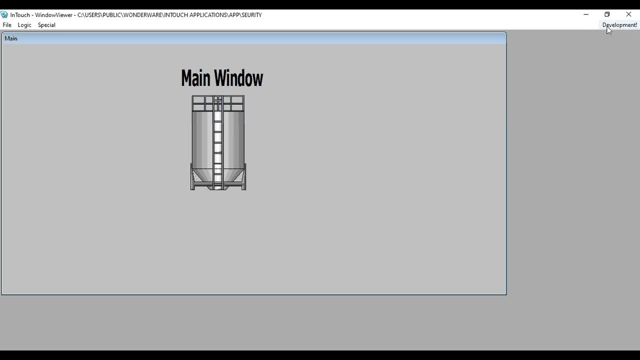 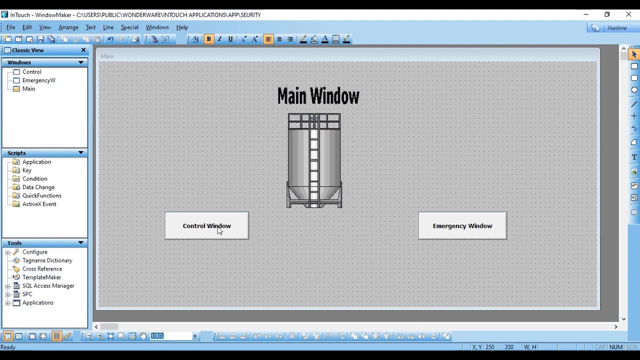 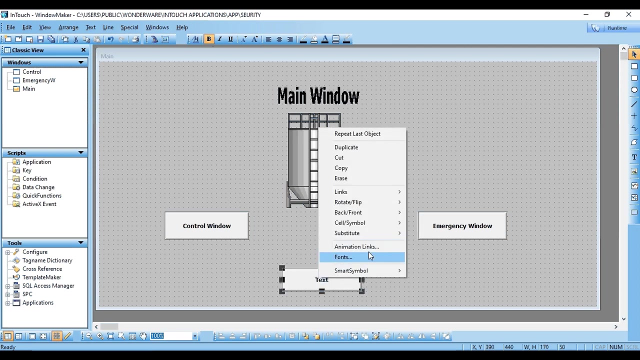 So hope you understand. So we can maintain any of the functionality using access level. the only requirement is we need to login and match the access level. We can also use the operator function. let's check. I am just adding a button. Let's say shut down, and we are adding this to shut down entire plant, just for demo. 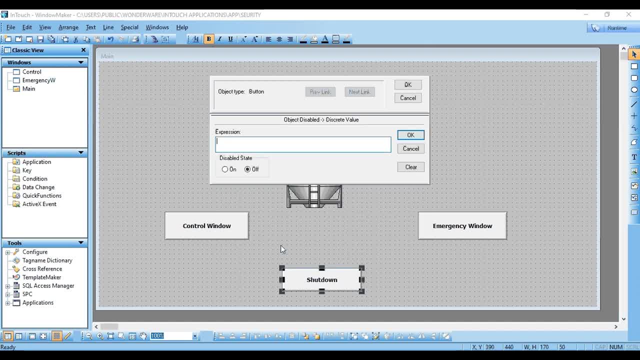 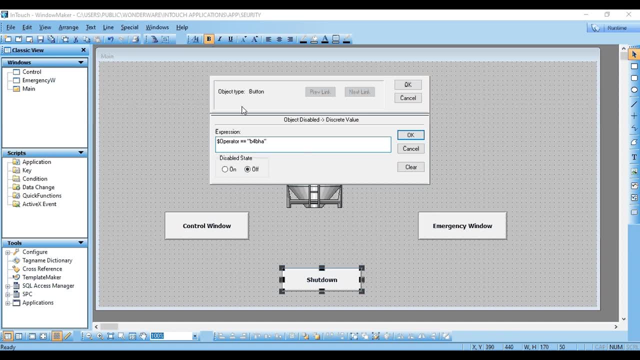 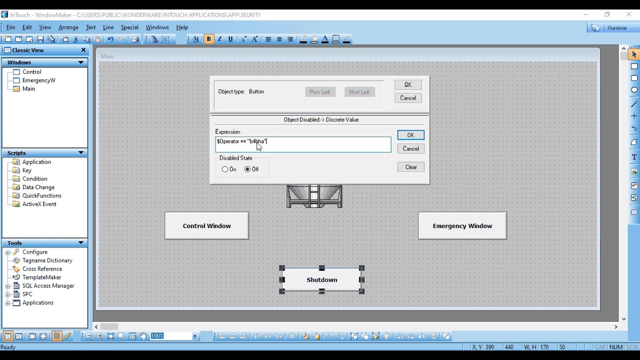 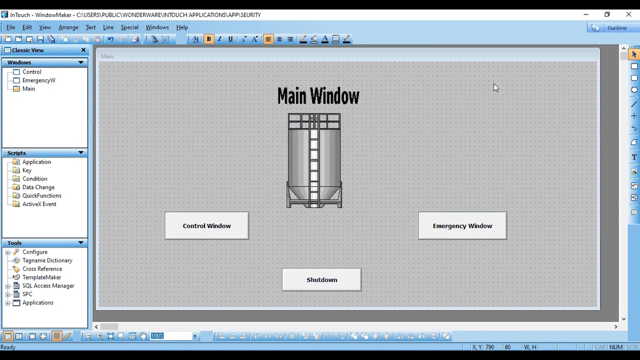 So I am adding disable functionality. So if I am adding it to disable function, If the dollar operator is equal to B4BHA, then only this button will enable. okay, otherwise it should be disabled. So let's check very quickly.